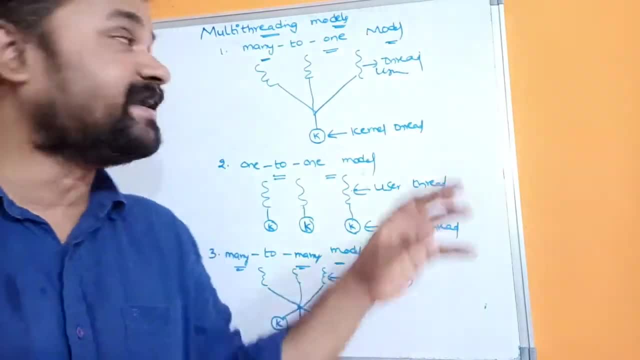 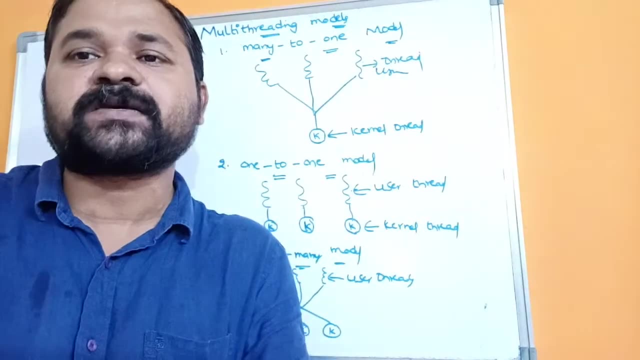 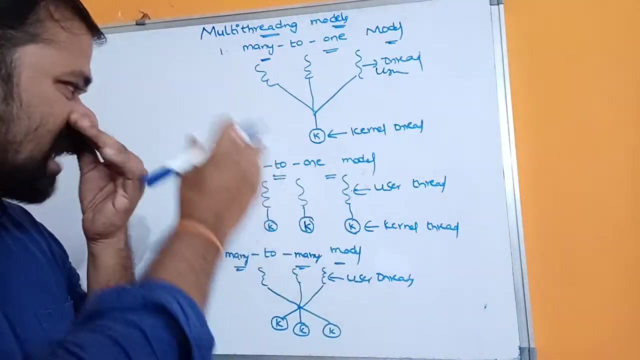 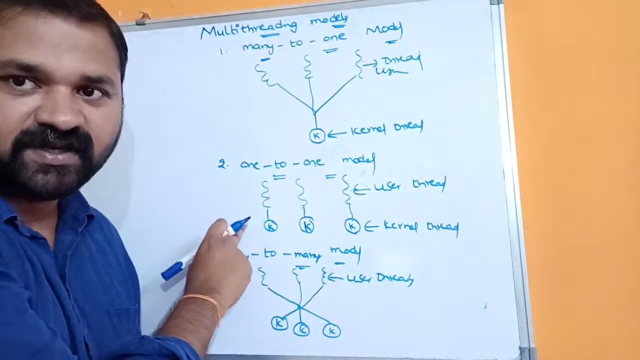 So one to one model solves the limitation of many to one model. The limitation of many to one model is it doesn't implement multi-processor architecture, So it doesn't implement parallelism, concurrency. Whereas, coming to the one to one model, here each user thread is mapped to a separate kernel thread, So this is thread one. So for this thread, one is mapped to this kernel thread. 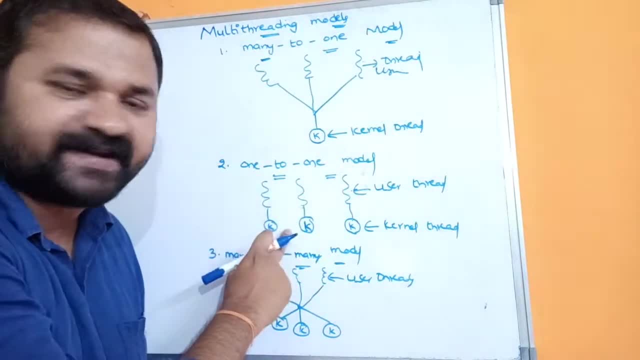 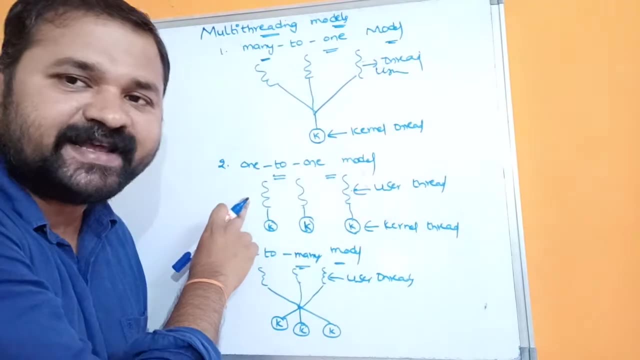 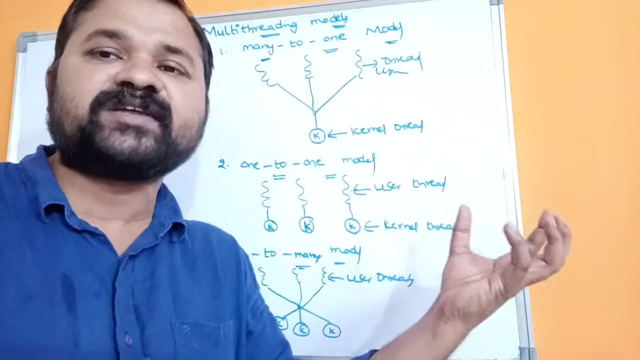 So this is thread two. So this thread two is mapped to this kernel thread. So this is thread three. So this thread three is mapped to this kernel thread. So if one thread is blocked then there is no problem. Why? because the remaining threads can access those corresponding kernel threads, So the remaining user threads can be executed by the CPU. 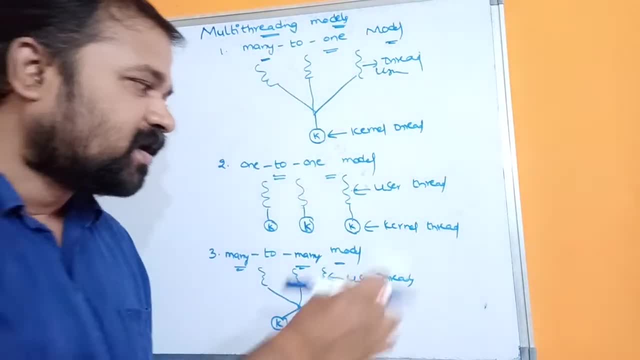 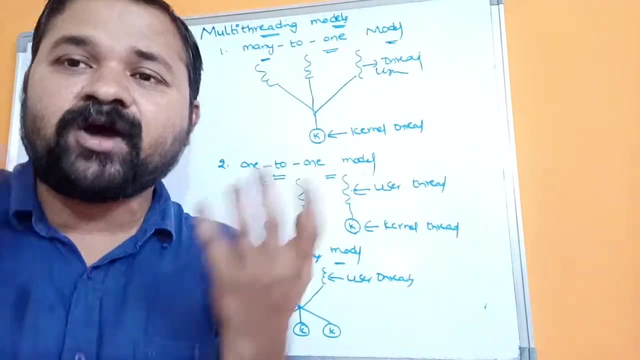 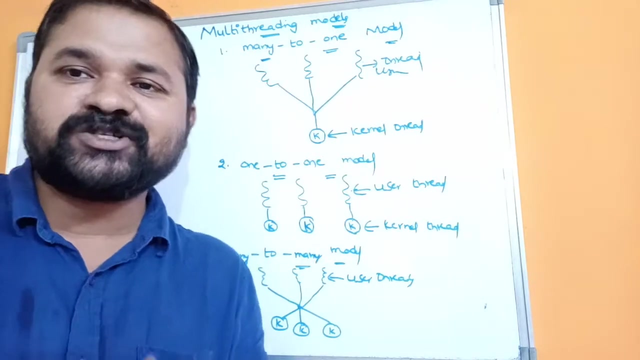 The major problem with this approach is the number of kernel threads which we want to create. If we create more number of threads, Then it is a burden on the computer, So the performance of the computer will be decreased, Will be reduced. Let us assume that in order to execute a process, we have created 20 threads. 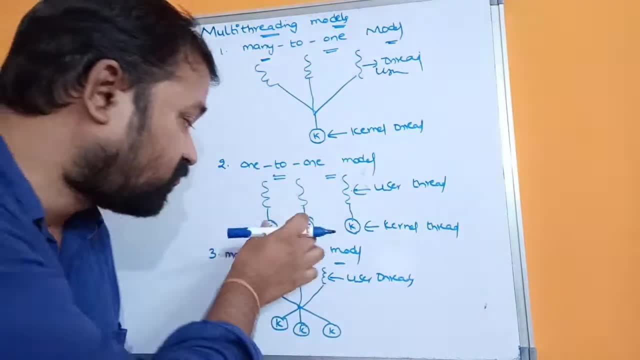 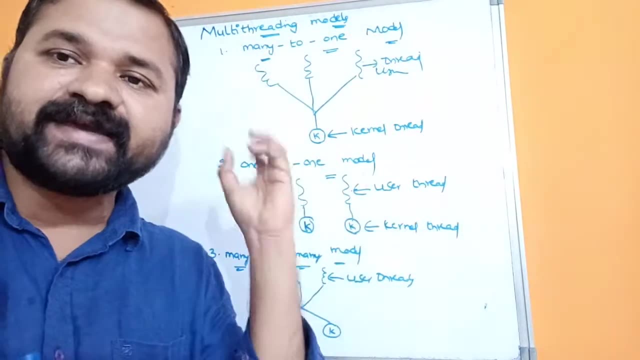 So for 20 threads we need to create, For 20 user threads, we need to create what? 20 kernel threads by the operating system. We know that operating system creates kernel threads, Whereas these user threads are created by our process, our application. 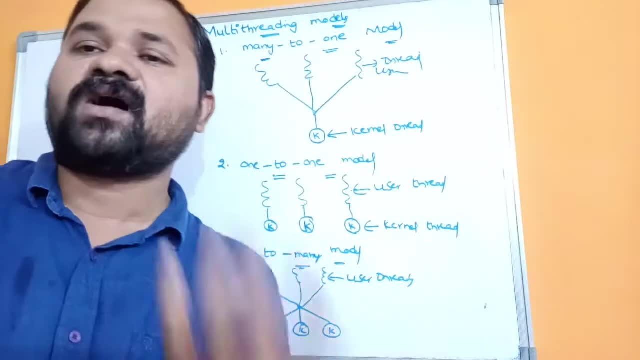 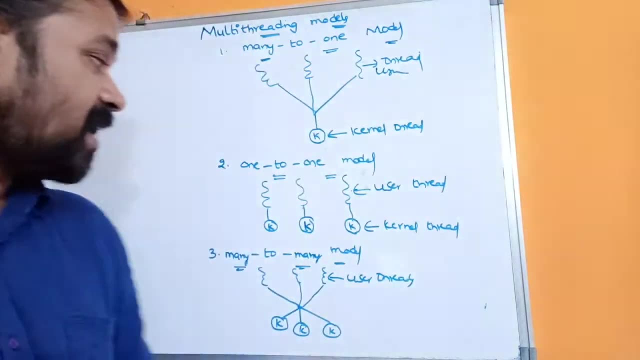 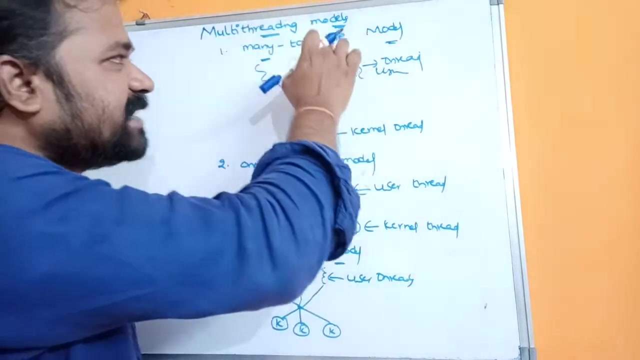 Okay, So 20 kernel threads are created by the operating system, So it is very, very burden on the computer, So the performance of the computer will be reduced. In order to solve these limitations, we can use many-to-many model. Many-to-many model solves the limitation of many-to-one model as well as one-to-one model. 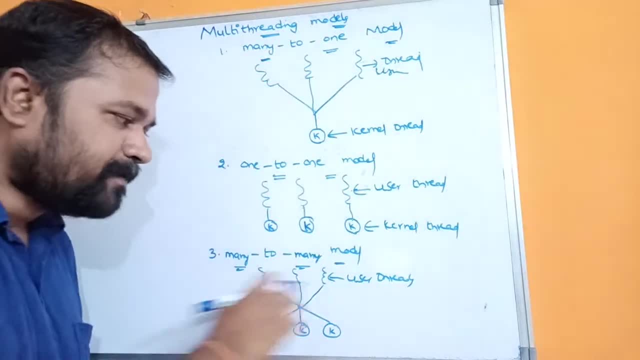